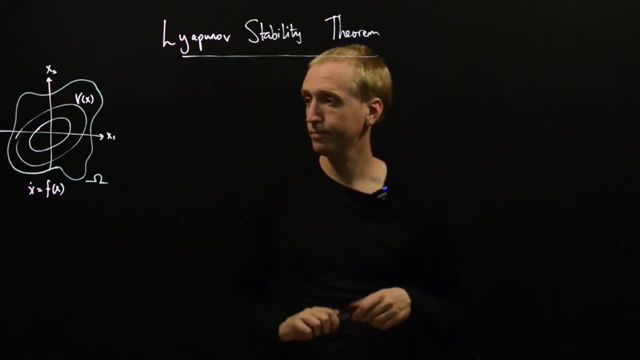 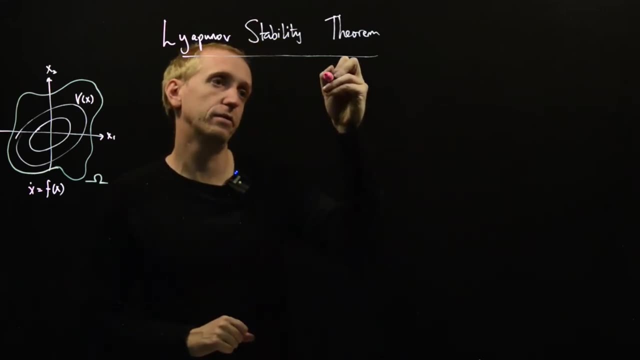 consider some different ones. So what are the set of Lyapunov stability theorems? Well, I just start to write them out, and so what we're going to be dealing with is we're going to say: we're given some non-linear system: x dot is equal to f of x. 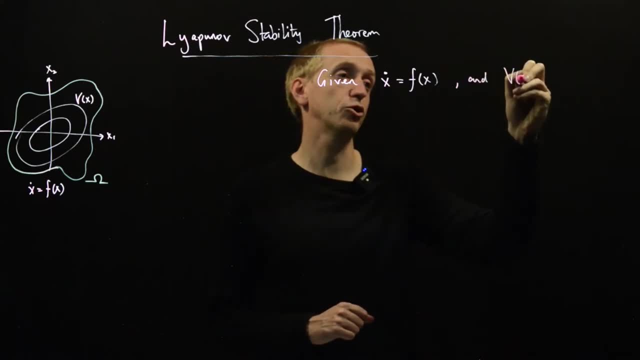 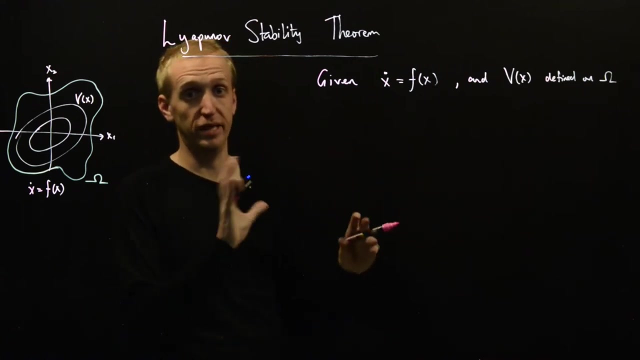 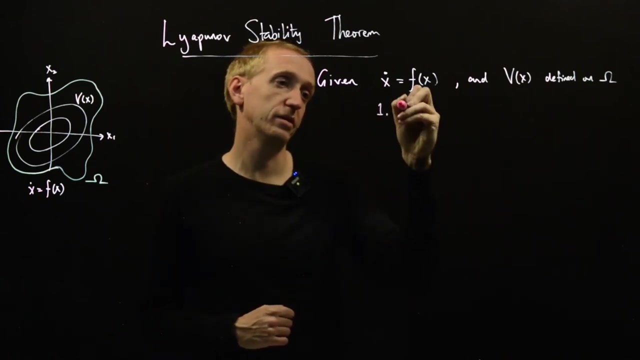 and we also have some Lyapunov function, v that is defined on on our region of the state space omega. Now, what conditions do we need in order to be able to make some conclusions about stability? Well, the first thing that we need is that v of x is equal to zero. 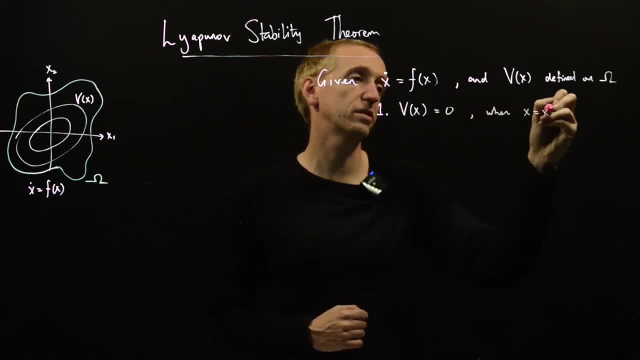 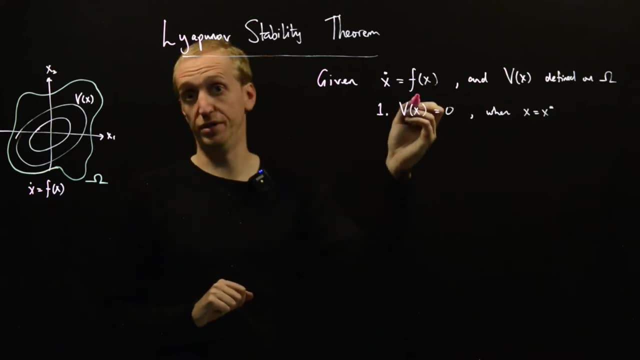 when x is equal to x star. So this is just saying that the value of our Lyapunov function at our equilibrium point, which on this picture is at the origin, is equal to zero. The second condition is that the value of our Lyapunov function 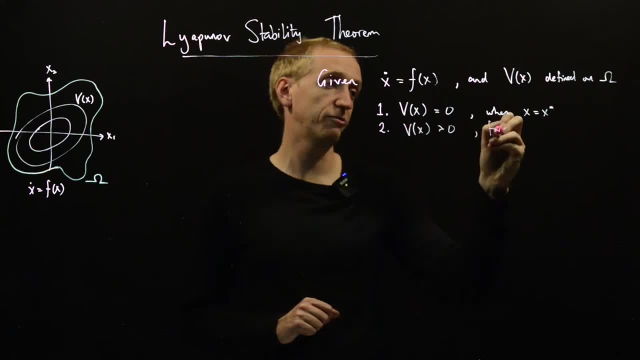 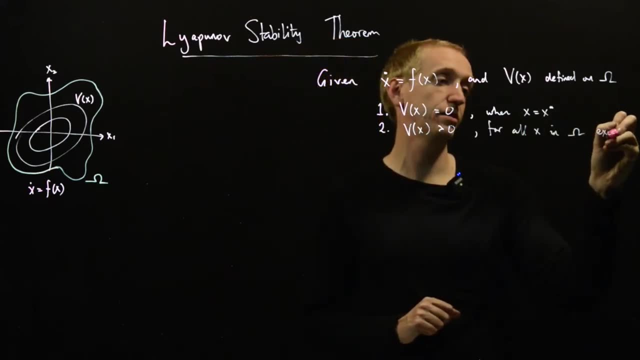 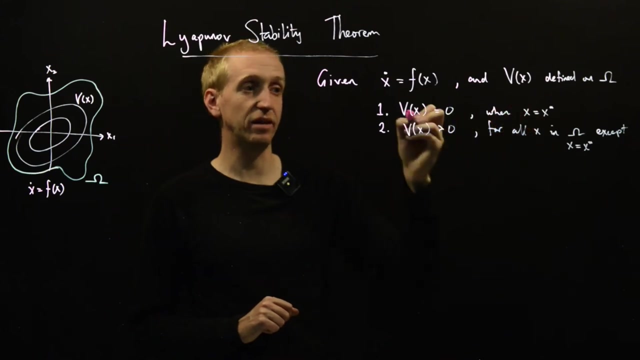 is larger than zero, and this is for all x in omega, except x, is equal to x star. So we've said that at x star the value is equal to zero. It needs to be bigger than zero everywhere else in our region omega, which must also include our equilibrium point. So these are our sort of two basic. 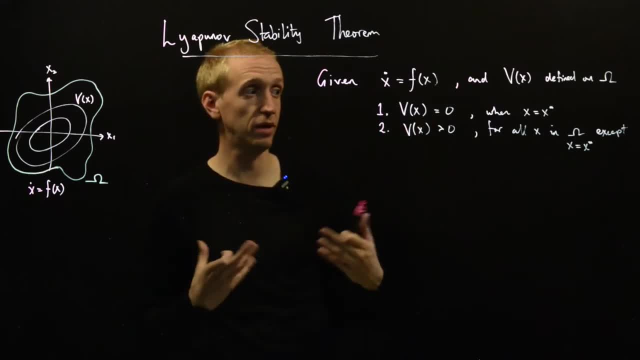 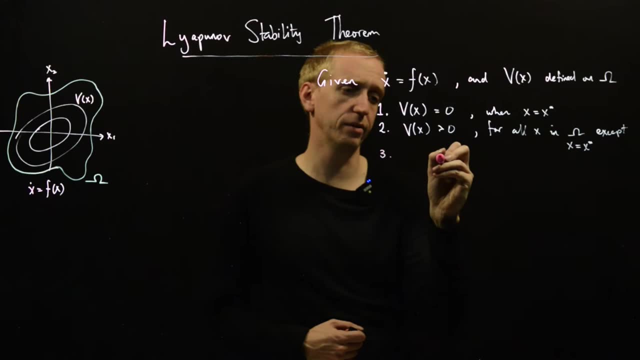 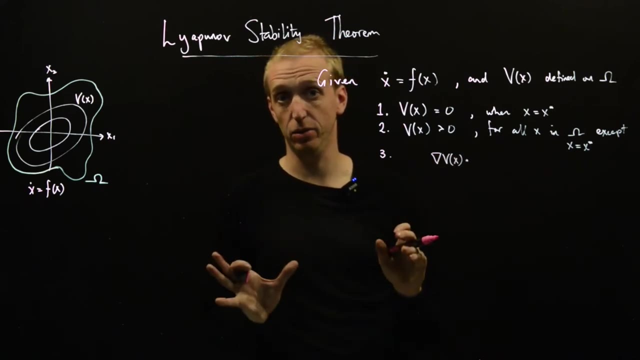 properties for Lyapunov, Lyapunov function that we saw last time. and then we argued that if something involving the gradient of v, when we take the dot product with x dot, and so what is x dot? well, x dot is just f of x. so if we look at the dot product, 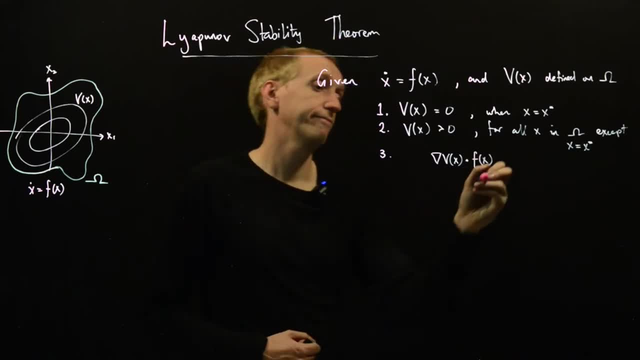 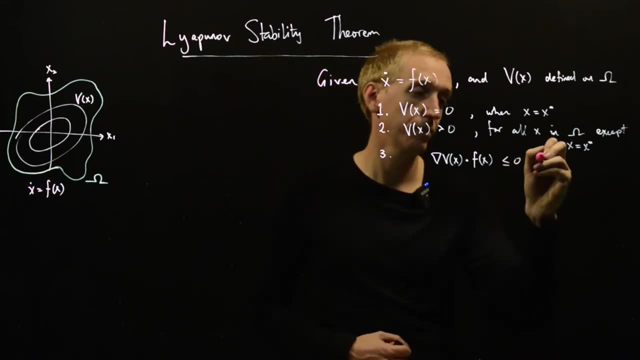 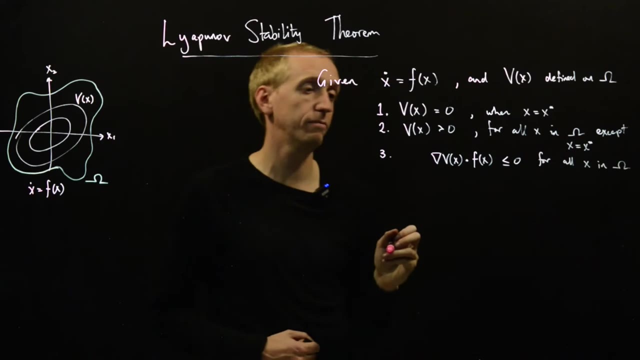 of the gradient to v with x dot if it's less than zero, less than or equal to zero. we have this i over x, dx and our result is that v in x star is less than zero minus zero times for all x in omega. this implies that x star is stable, and remember that stability was our weakest. 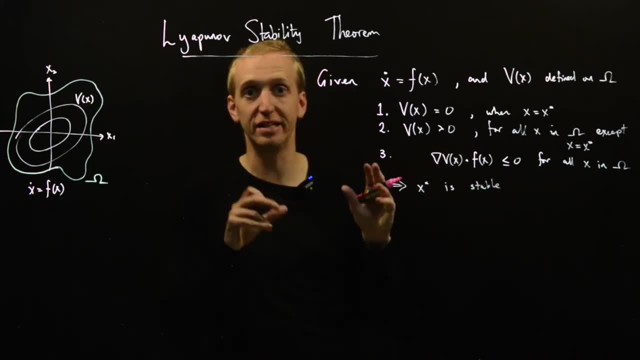 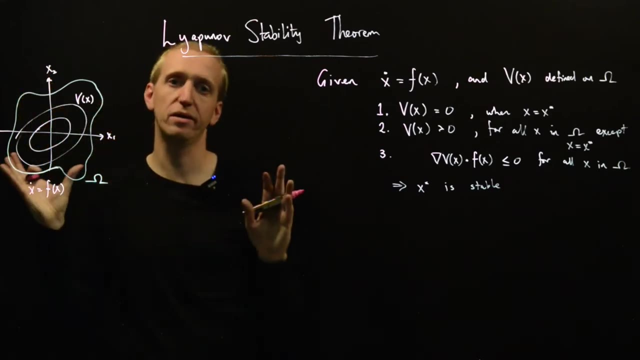 the stable was our weakest stability notion. We got the ideas of asymptotic stability, and global asymptotic stability was what we wanted to prove stronger. And all this means more formally is that if we start in this region, omega, we're gonna stay there. So why have I left a space here? Well, this: 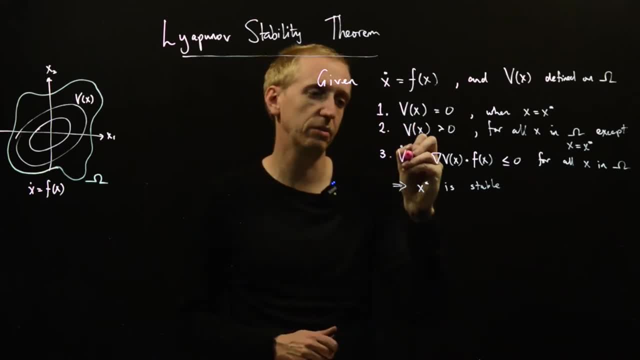 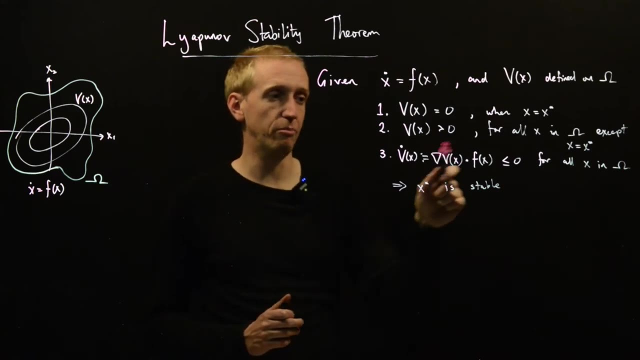 thing is often given its own name, and so V dot is defined to be this dot product here. So these are the conditions for stability using Lyapunov functions. and if you remember, here this was just corresponding to well, grad V was just. 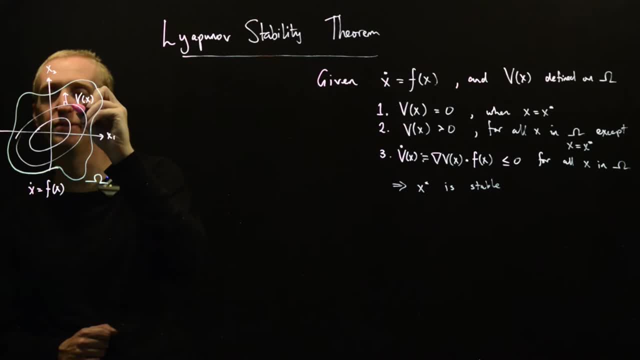 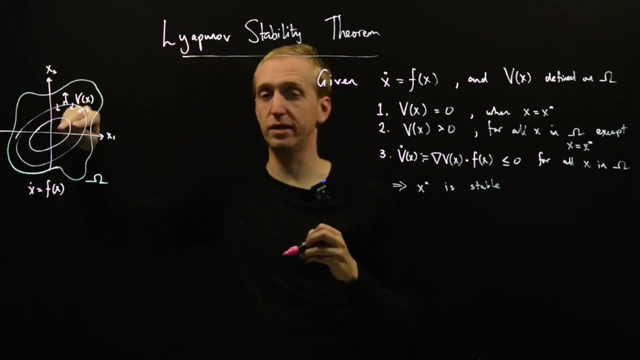 these vectors that were tangential, which are perpendicular to the level curves of the Lyapunov function. If I dot product those with my directions for x dot. well, if this is negative, it just means that we're moving to the contour of lower energy. So being less than or equal to means we could be. 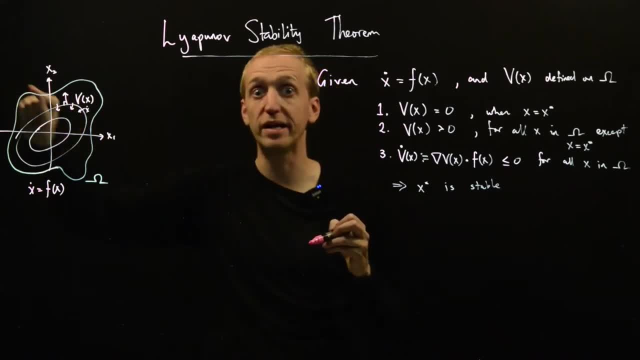 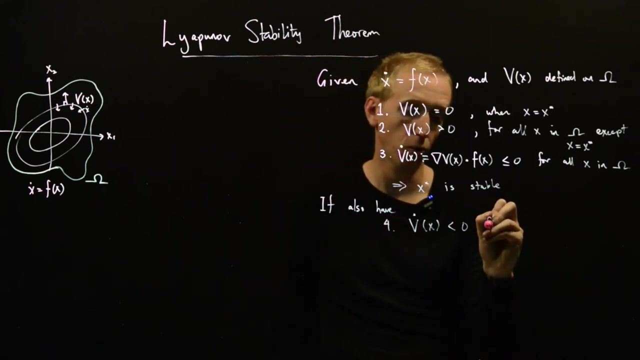 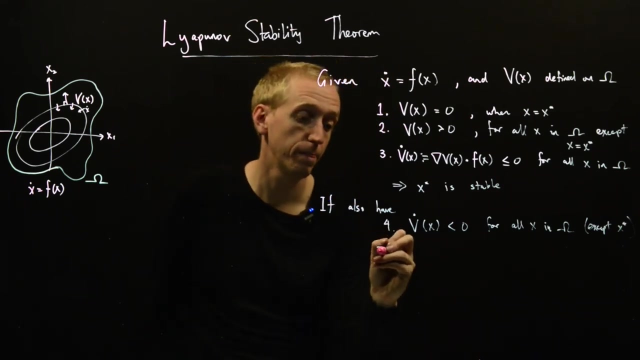 moving along the contour, but we're never moving away and getting further away from the equilibrium point. And so how does this get strengthened? Well, if we also have condition four, V dot of x, dot x strictly less than zero for all x in omega again, except at x star, then x star. 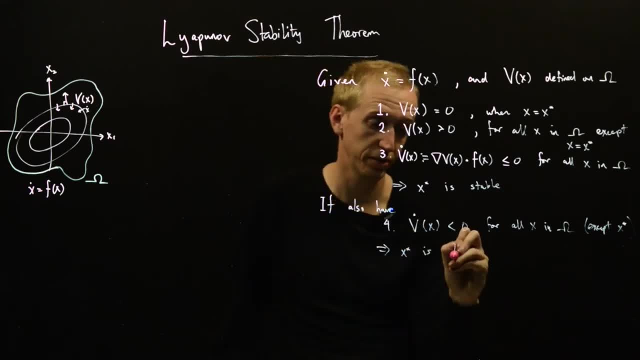 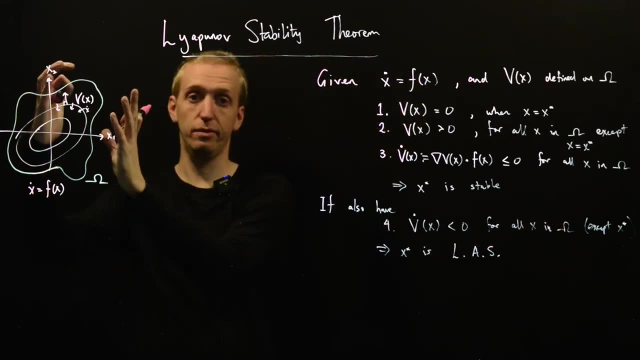 is locally asymptotically stable. So locally asymptotically stable and more than that. it's what this means is, given our region omega. if we start in omega, we will stay in omega and will converge to our equilibrium point, So we actually get a. 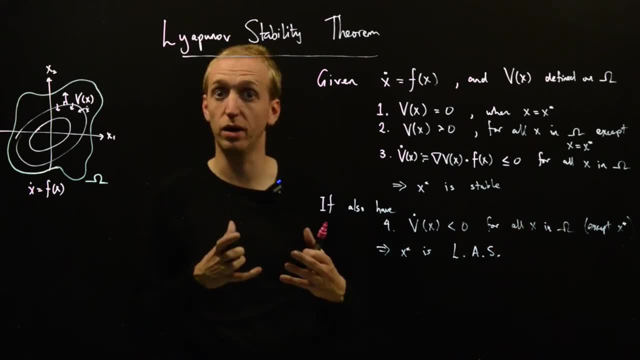 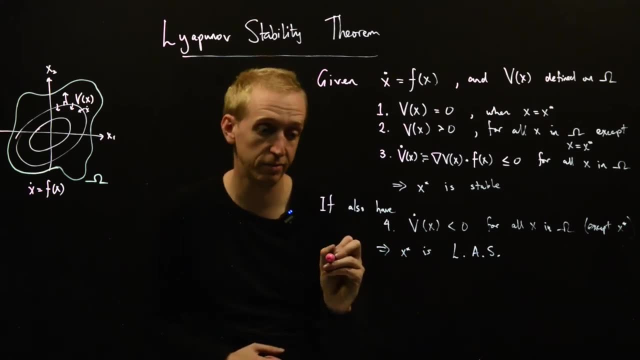 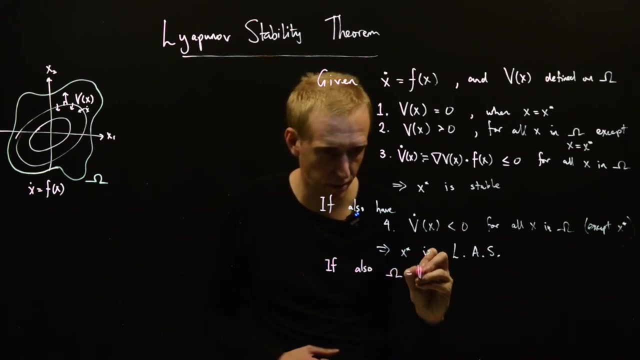 region of attraction coming with this through our Lyapunov function, And then finally we also have the extension to globally asymptotically stable. So if also omega is equal to Rn and this is just fancy language for saying that our region omega is the entire state space. So for all of this stuff here, 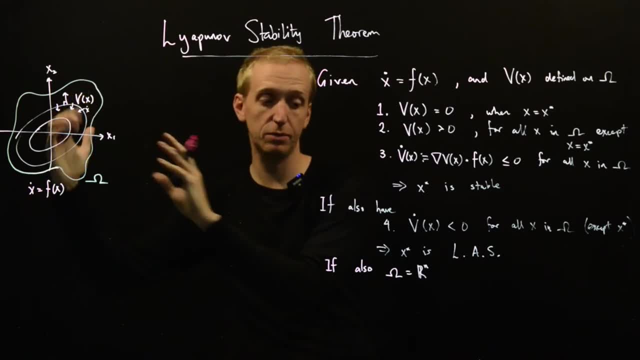 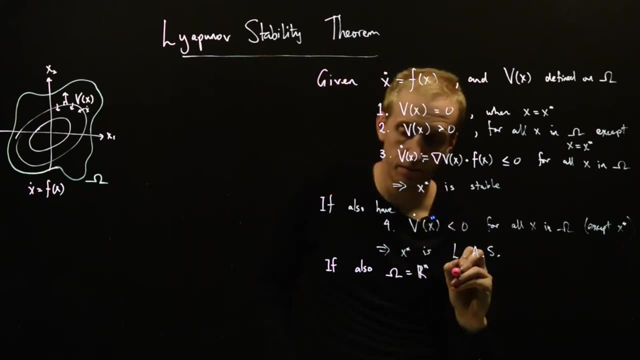 omega had to be some bounded region of the state space. We're now going to look at global extent And also so, if we also have this and v of x goes to infinity as the length of the vector x, which is just this square root of x1 squared plus xn squared, goes to 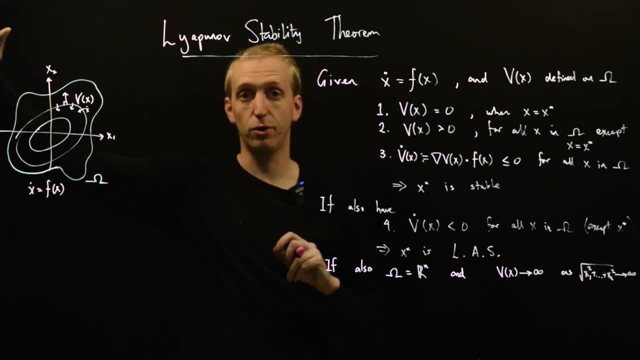 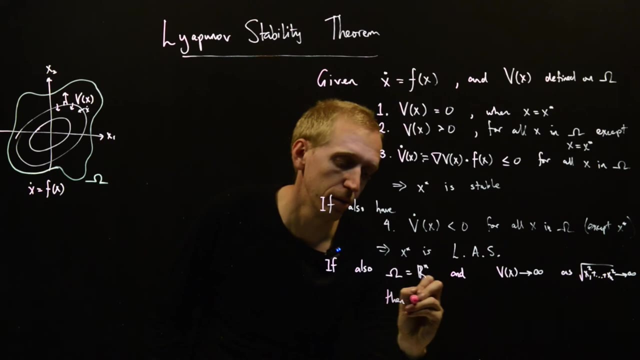 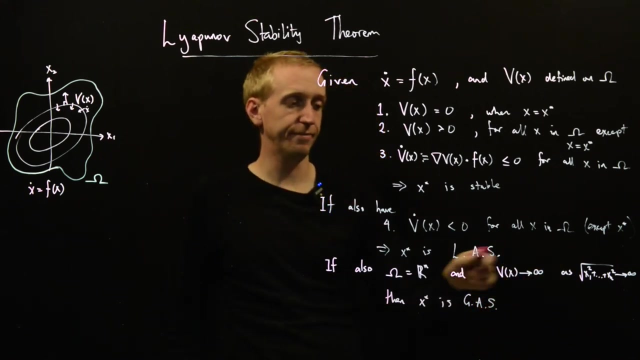 infinity. So as we move further and further away from the origin, we can see that the value of our Lyapunov function gets bigger and bigger and bigger and it grows without bounds. so if we have these things, then x star is globally asymptotically stable. This is a kind of an extra technical condition. 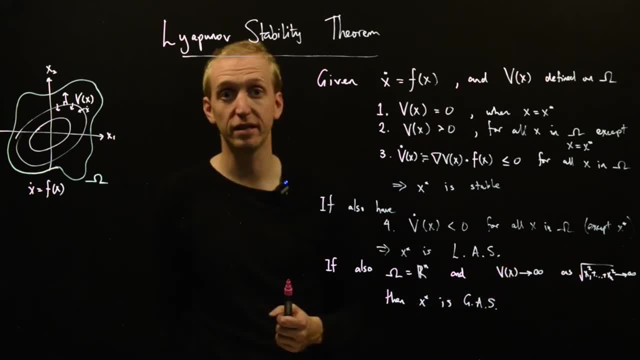 that's explained in a bit more detail in the lecture notes. I don't really want to get into it in too much detail. I mean, if you think about it, it's nice to be able to say that this system is globally asymptotically stable and in reality is not. it is actually good Music for learning to floating around at the bat. 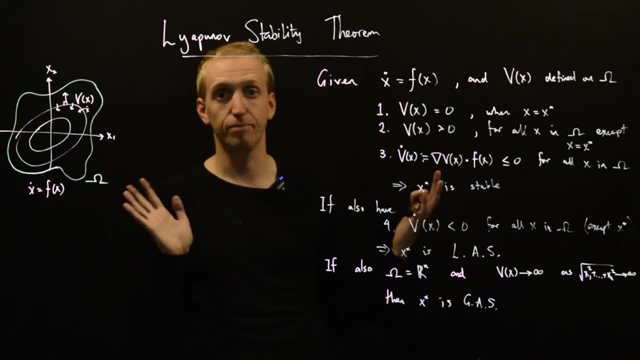 but a statement like this is actually completely meaningless in any physical way. So whatever space your system is going to be living in, it's going to be bounded. We don't often worry about the evolution of systems in the context of their behavior in the entire. 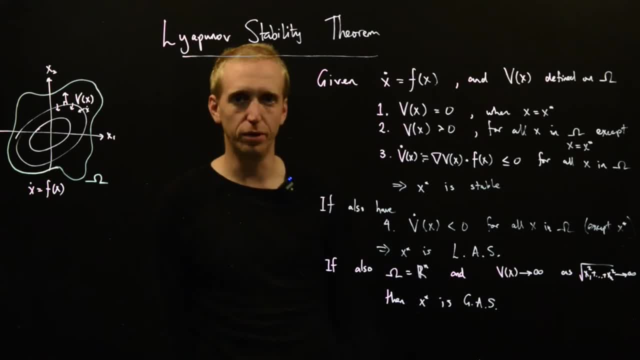 universe, and even if we did, it still wouldn't be truly infinite. So this is kind of like a nice little mathematical extension, And there's an example showing why you need this condition in the lecture notes. So here you have it. These are our Lyapunov.